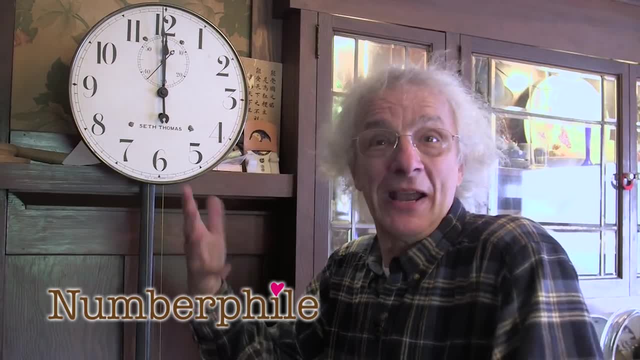 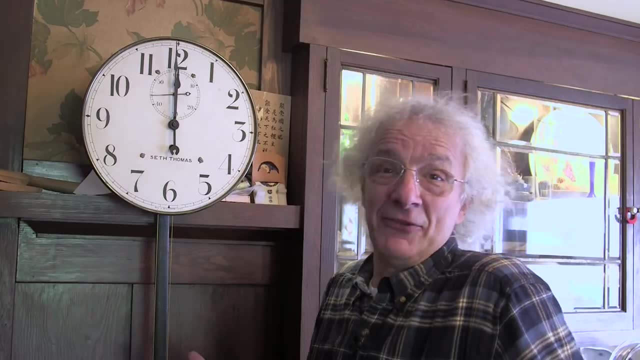 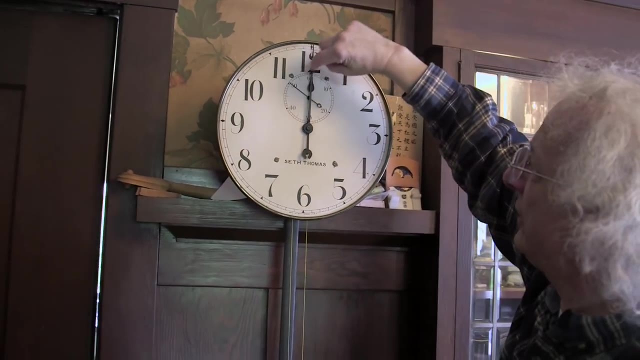 It used to be that clocks had faces on them. They're analog clocks. They're unknown today. but you know, occasionally you find one And you look at it, you have an. at least I have an immediate question of: hey, if it's noon, how long will it be? you know these are lined up. how long will it be until they're lined up again? 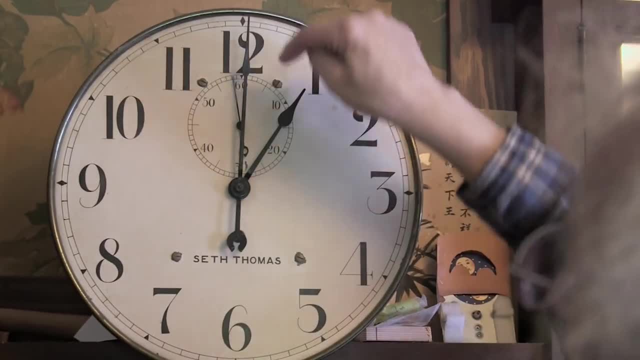 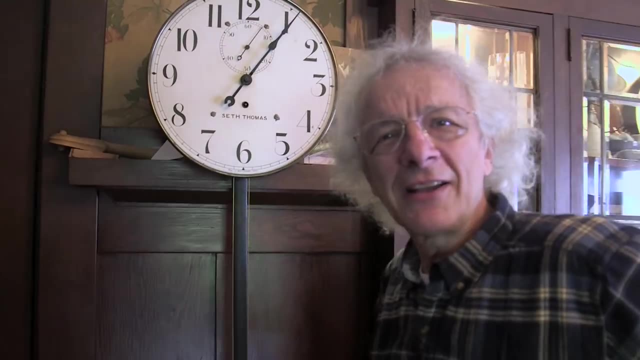 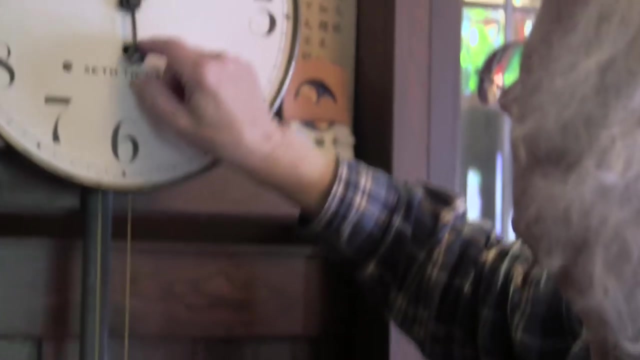 Well, not, it's more than an hour, but you know how long. until you know just at exactly what time will the clock hands line up? Okay, a little bit after one it'll line up, and line up again a little bit after two. 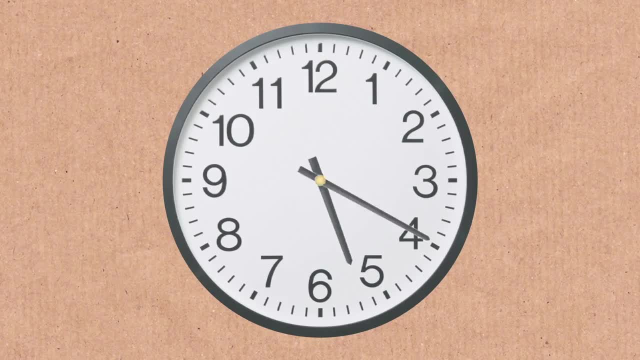 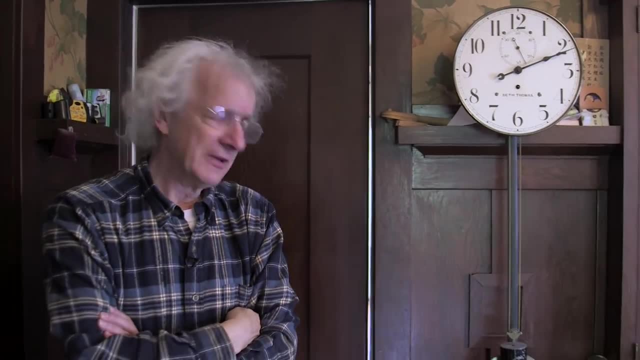 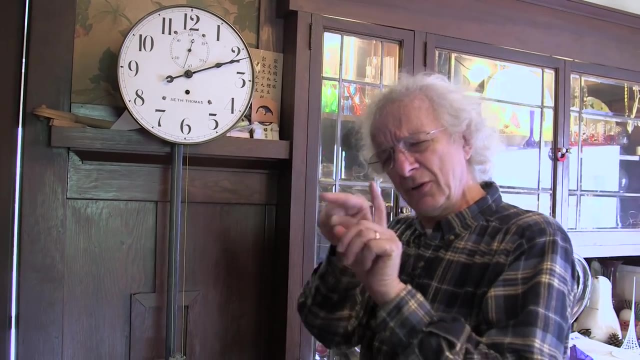 So what's the time difference between there, You know, and you say, well, it's more than an hour. How can I figure that one out? I'm sitting there saying, you know, I remember, I remember sitting in a fifth grade classroom trying to figure it out, drawing diagrams and thinking, boy, I need to add a little bit more, a little bit more. just, it's going to be a little bit more than that. 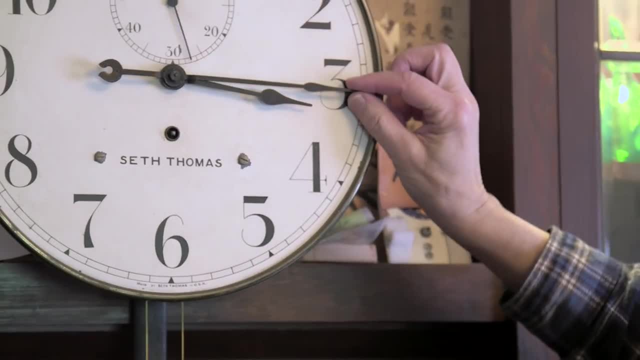 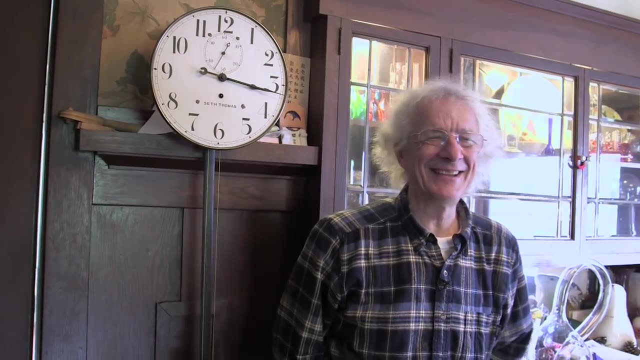 It's going to be, and then you know it's going to be more than that. more than that, How much, how much time until? and then, like you, I realized: oh, there's a simple way to solve it. 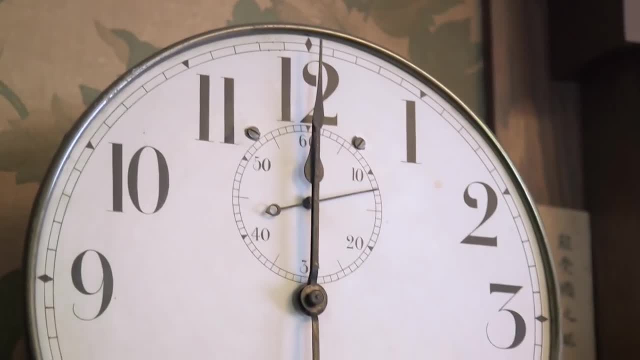 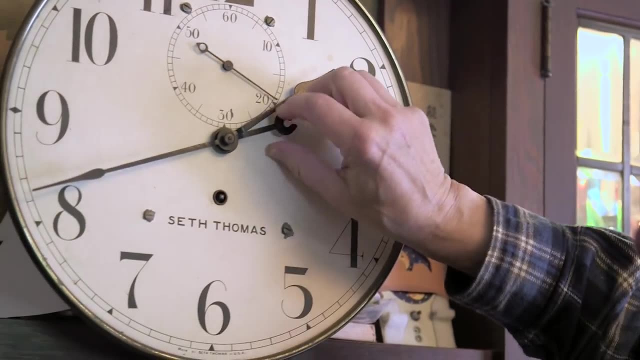 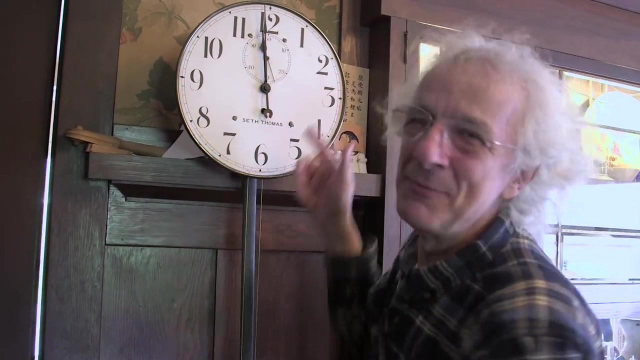 Let's go back to noon. How many times do these hands cross in 12 hours? Well, there's once, twice, three times and so on. In fact, think about it and you'll realize: the hands cross each other 11 times every 12 hours. 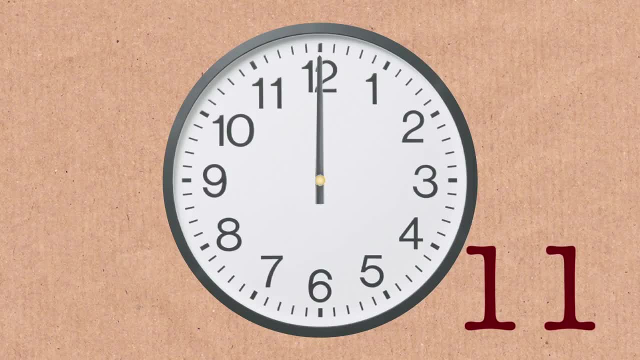 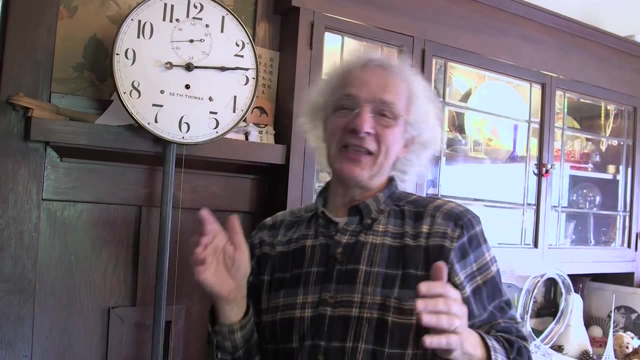 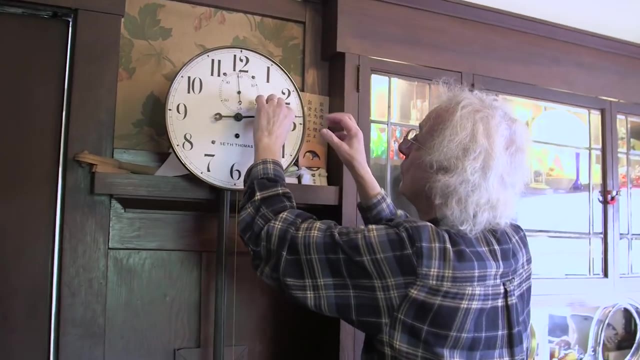 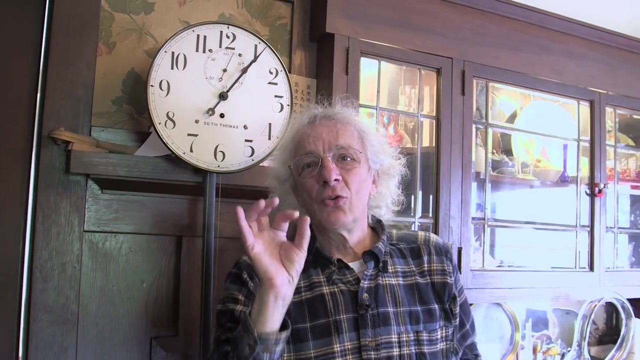 Ah, if there's 11 hand crossings every 12 hours, that means that they will cross each other. So that means how long will it take for between here to here? That must be 12 divided by 11 hours, which happens to be.